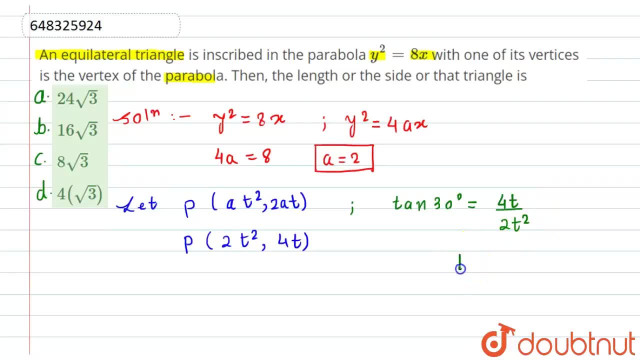 So, on solving What we get, we get the value of t will be equals to 2 under root of 3, because tan 30 is what you can see here. this 2 to the 4, 1t, 1t will be get cancel out. t will go to that side, while this 1 upon under root 3 will come to this side. 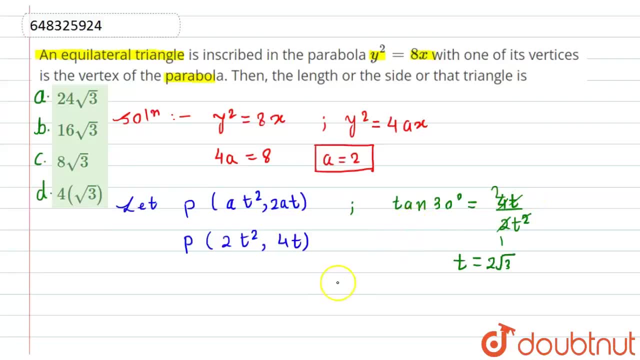 So become 2 under root of 3, because tan 30 is nothing but 1 upon under root of 3.. So here we got the value of t on substituting here our point p Will become how much that is under root. 3 square will become 3, a 2 square will be 4, 3, 4 is a 12, 4, 12, 4. 2 is a 24 comma and similarly this point will become 8 under root of 3.. 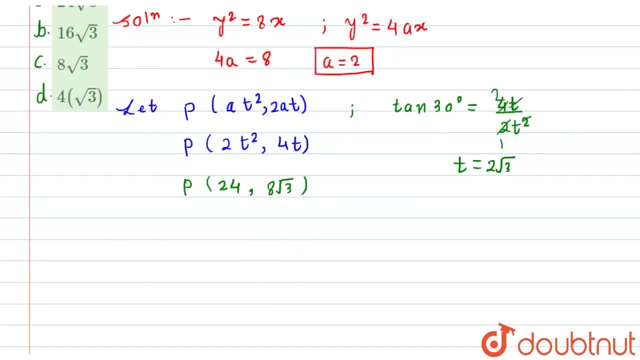 Now, here we have found a point. now, simply by using distance formula, I can able to find the length of the side of the triangle, that is, we will say the length of side Of triangle. it will be equals to Under root of 0 minus 24 into square, that is 24 square. 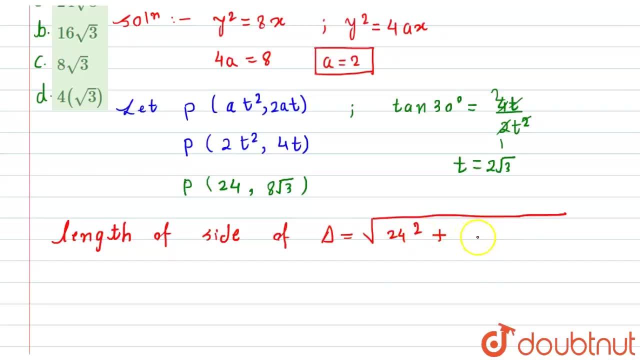 Plus 0 minus 8 under root of 3 square, that is 8 under root of 3: 8 square. So this will equals to root over 24 square. is how much 576 plus now 8 square 64.. Okay. 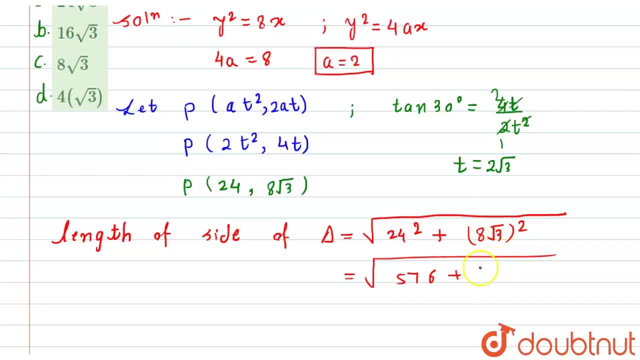 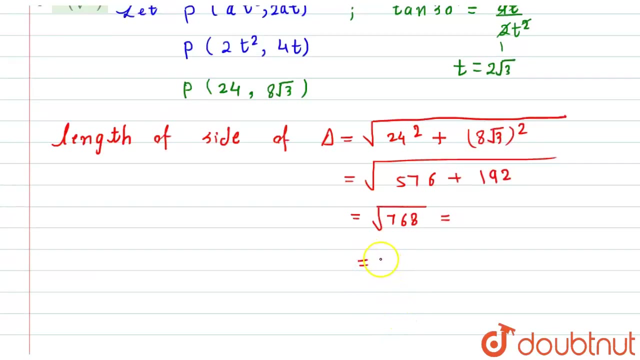 Okay, Okay, under root, 3 square will be 3,. 3 multiplied by 64 will be 192.. On adding you will get 768.. And on further solving this value will become equals to how much That is 16 under. 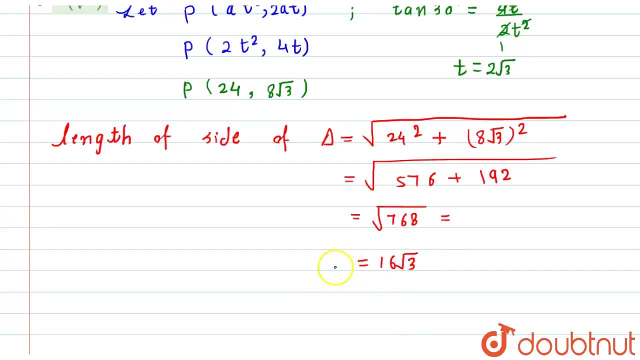 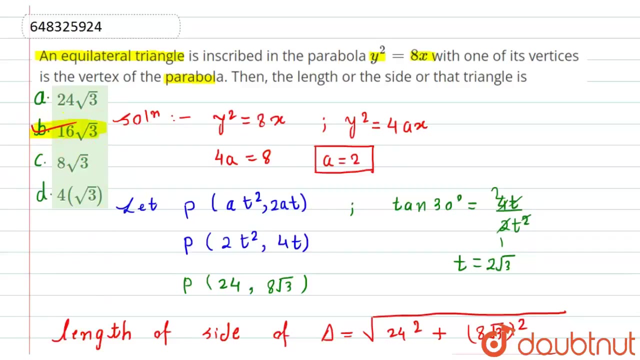 root of 3.. So we got the side of the triangle is how much That is 16 under root of 3, and this is what our required answer. Now let us take option here. So option B will become correct. So this is the required solution, Thank you.